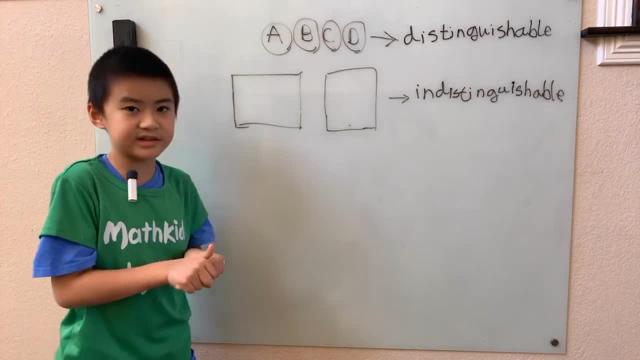 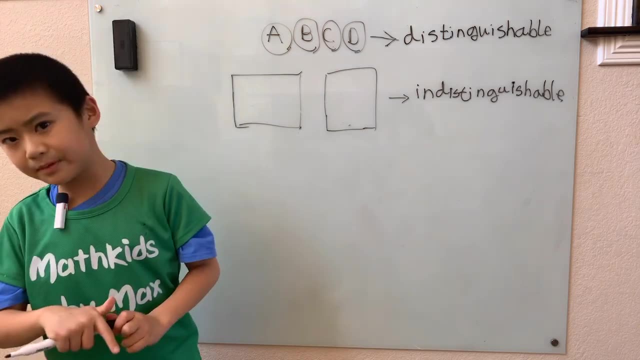 that all the time. So the stupid way we're going to do here to solve this problem is by using casework, And if you didn't know about casework, casework just means there's some things that could happen and we count how many ways. 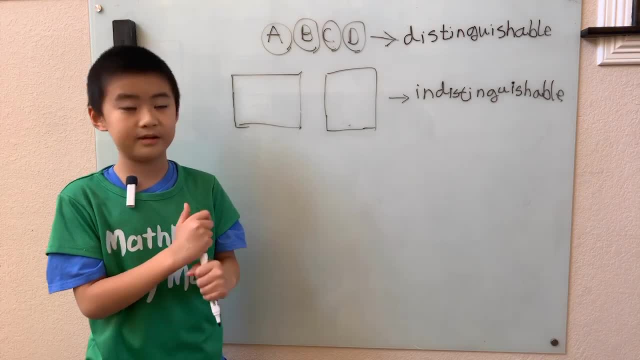 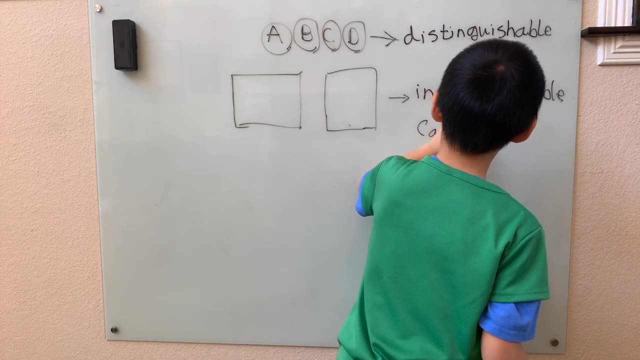 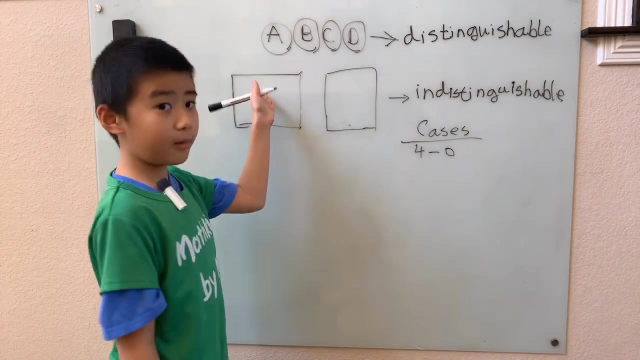 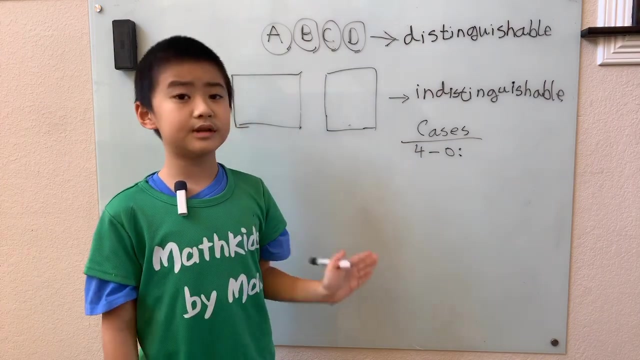 We could, how many possible different ways would happen if one of those cases came true? What this means is, if I have the balls arranged four to zero, meaning four to zero, meaning four balls in one box, zero balls in the other box, if this is true, that's one of our cases. 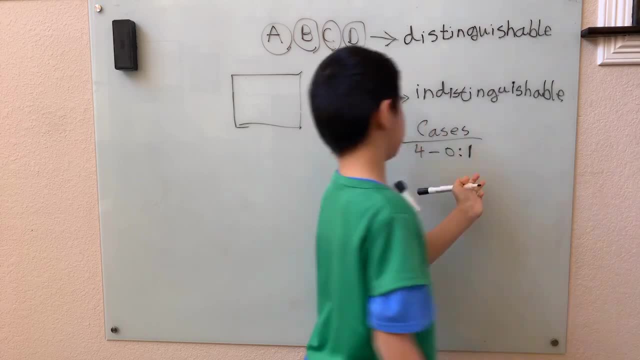 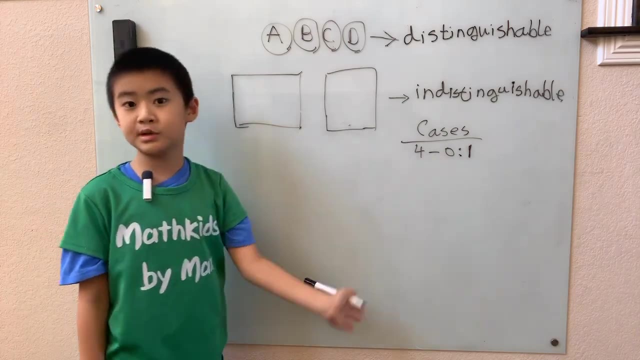 if this is true, then that means there's going to be one possibility. If we make it four to zero, it's true, But note that zero to four is the same thing as four to zero, because we don't care where the four balls are, because these are indistinguishable. 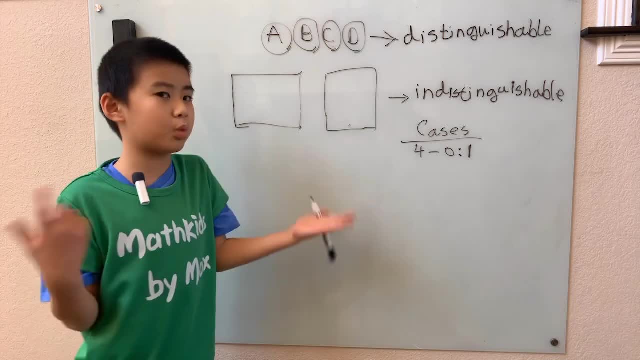 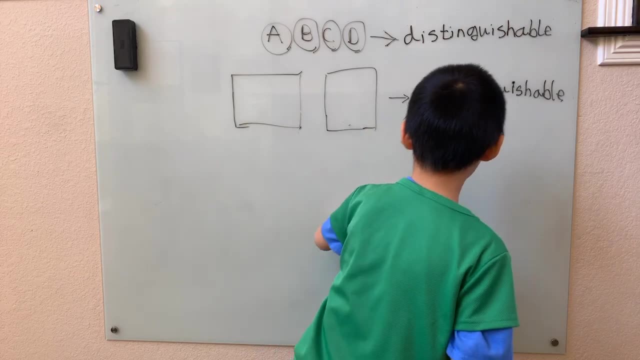 boxes. They're the exact same boxes. We don't care where the balls are, We care about what they are. So now we've got two more cases to consider For area one. we're going to consider that first, and then we're going to consider two too. 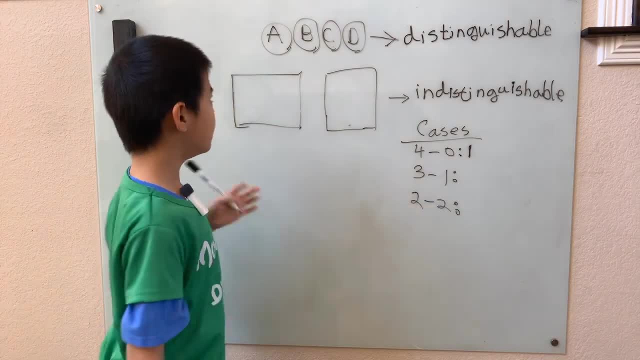 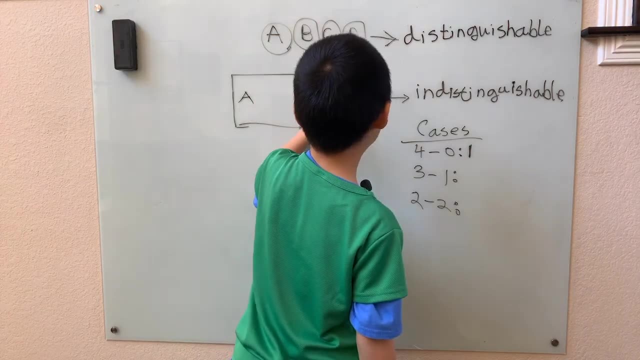 Where the boxes have the same number of cases, same number of balls. One of the possibilities for a free one is to have A being lonely, A alone, and B, C, D on the other side, And we can note that by this kind of diagram. 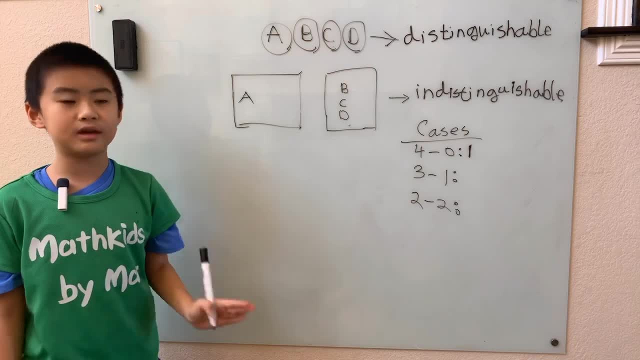 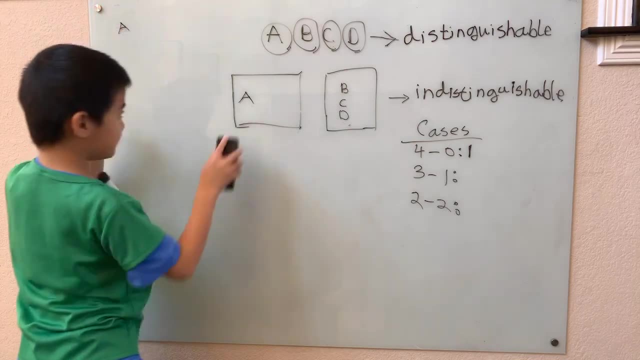 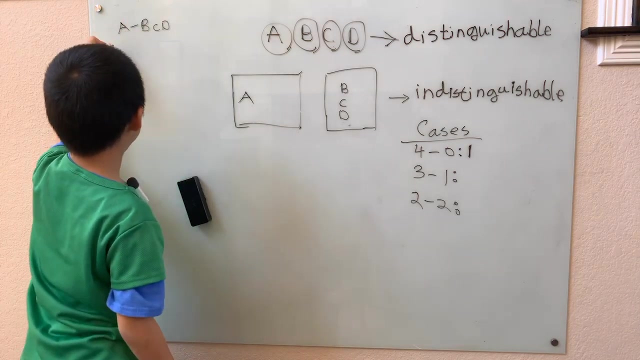 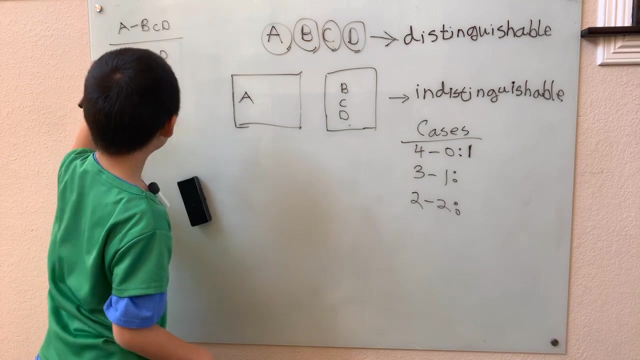 we know that there has to be at least one lonely little ball in one of these boxes So we can write down all those conditions. That could be A to B, C, D, the one we're showing right now, Or we could swap the A and B to get B versus A, C, D, And you can. 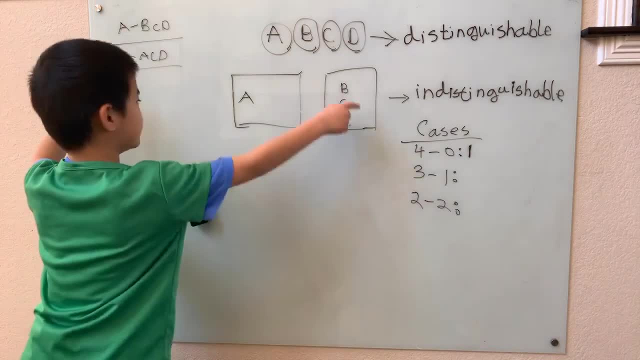 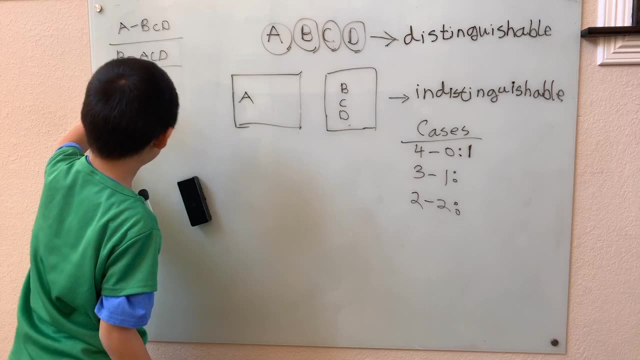 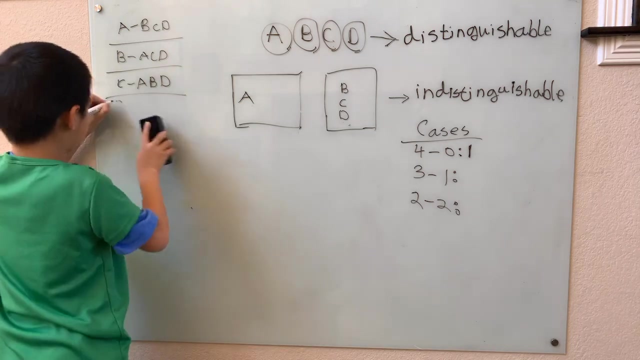 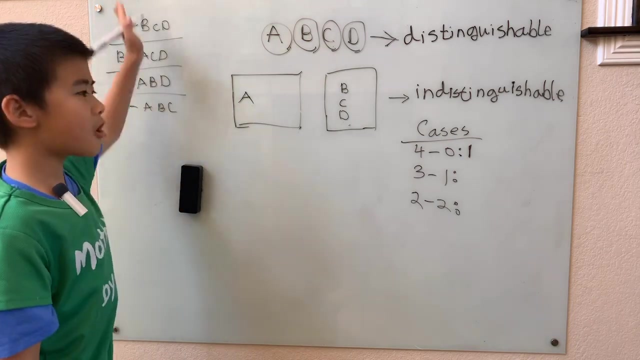 do the same kind of swapping thing for the other two, the C and D. Swap the C and A to get C versus A, B, D And last one, we have D versus the other three, A, B, C. And these will be our four combinations or possibilities when they have free one. 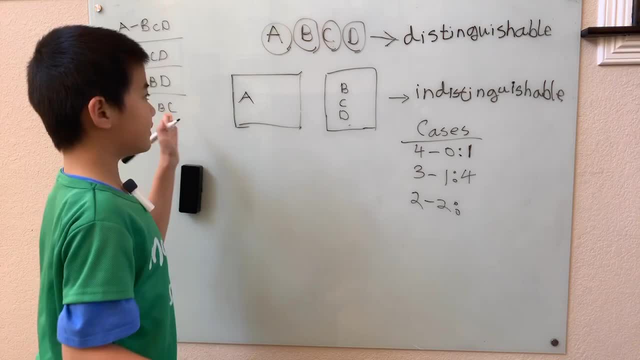 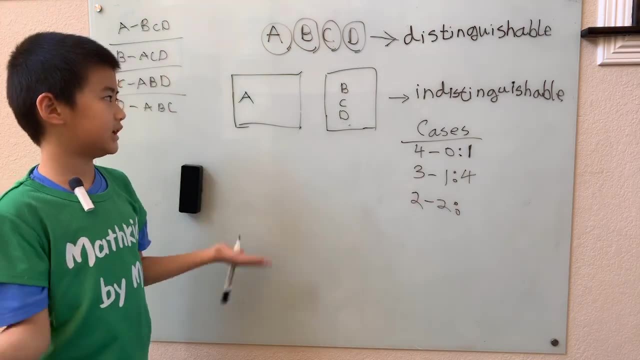 Because note again that if we move on, that if we swap these two, they're the same indistinguishable box. We don't care about where the balls are. So anyways, we move on to 2, 2.. Now 2, 2,. 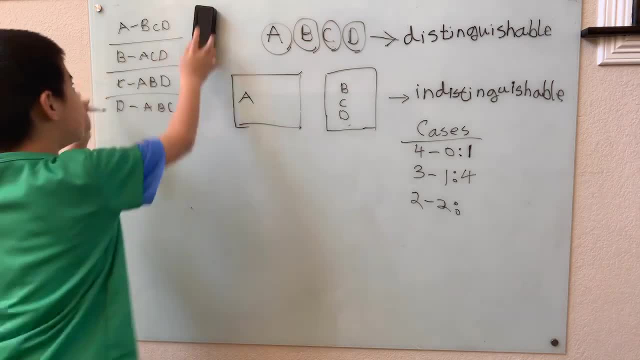 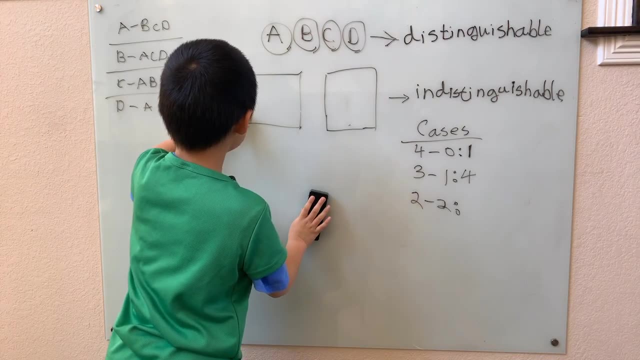 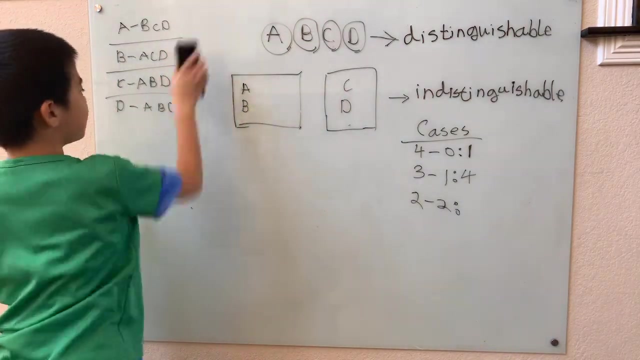 a little more complicated, But we'll use the same strategy that we did with the free one. We look at one arrangement and see that arrangement will be A, B versus C, D. So now we basically did the same thing. We look at what will happen if A stays in this box, if B stays in this. 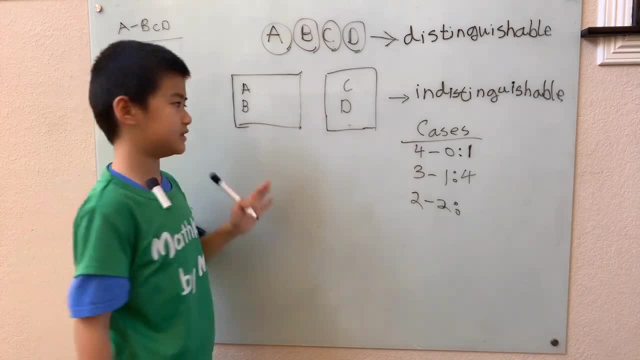 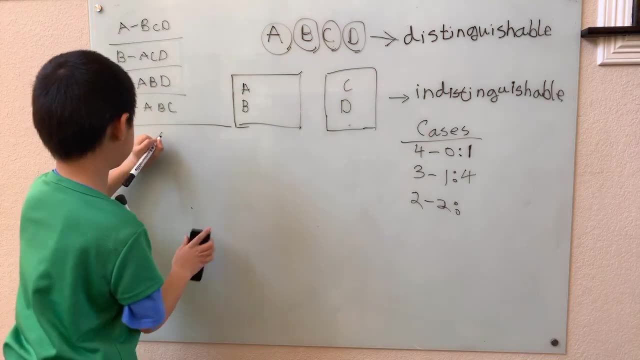 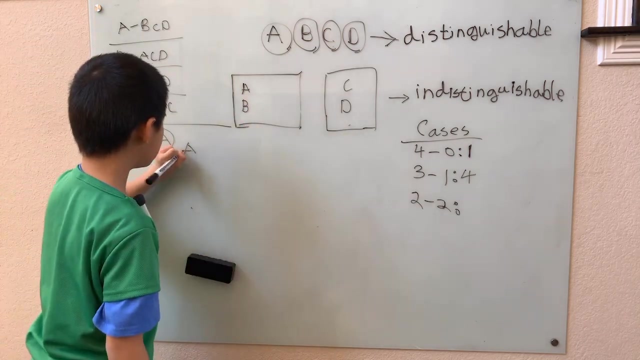 box, if C stays in this box or if D stays in this box. Now we first start with the A staying in this box. The A stays in this box And in this box where there's one combination- A, B versus C, D, the one we're showing. 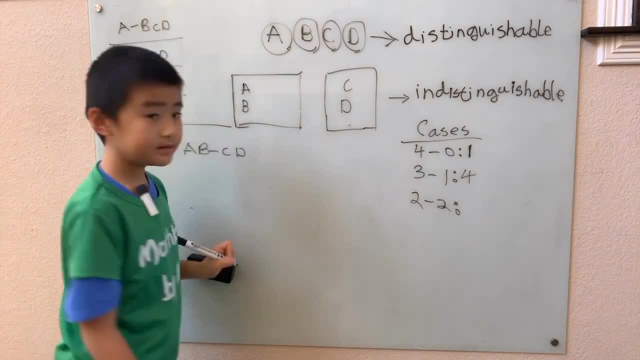 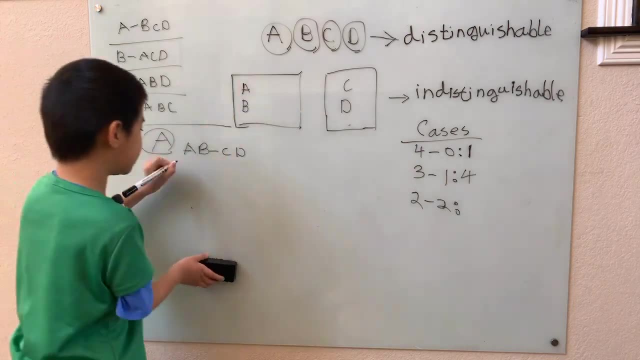 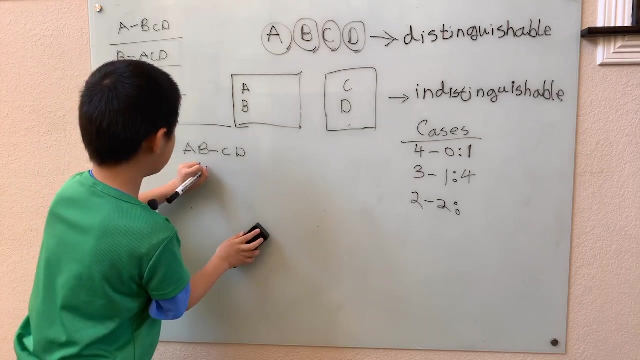 A, B versus C, D. And another one: we swap the B and C because, again, note that we want A to stay in this box. We'll have A and C, and C versus B and D, A, C versus B, D. And one last one: swap the. 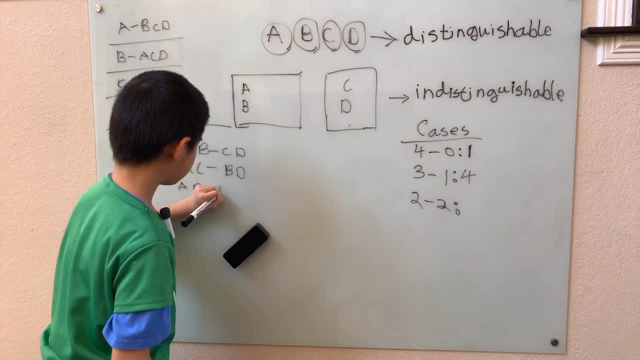 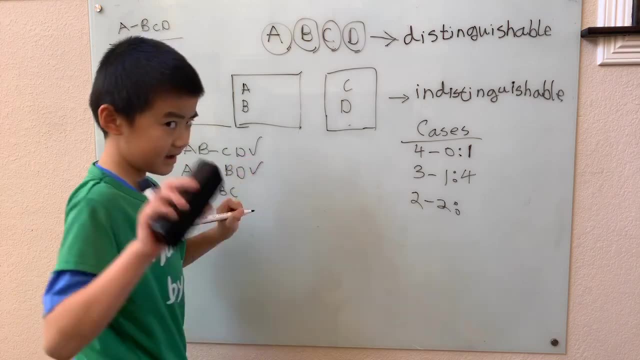 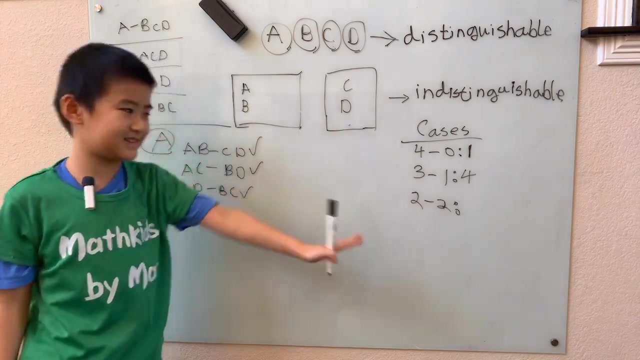 B and D, A D versus B- C, And since all of these are combinations that we had not counted before- and note that when I say had count, you can probably guess that there's going to be some possibilities that we already counted in here. you see what I mean. 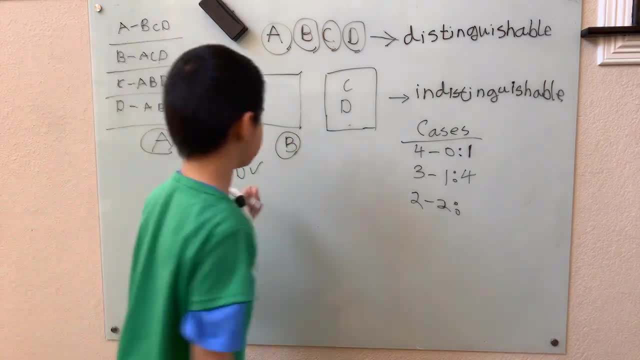 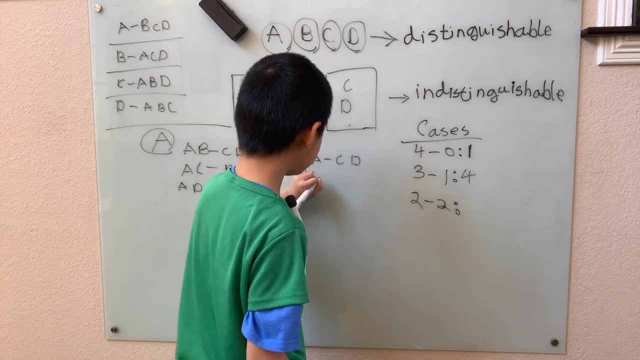 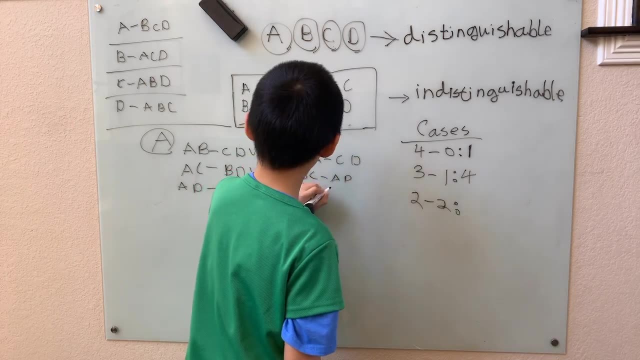 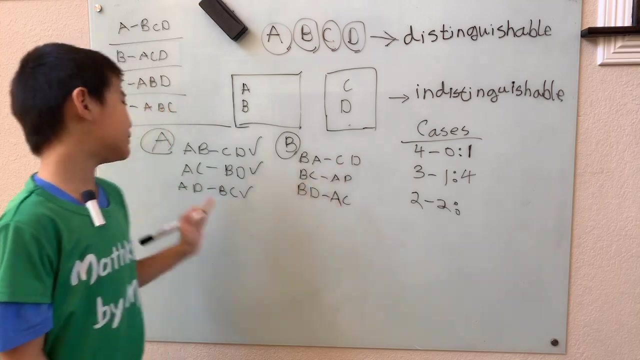 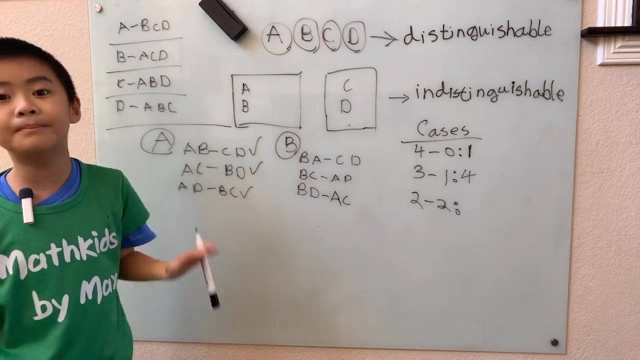 D. We counted A, A, B, C and D and we already counted that It doesn't matter that these two are different, that we swapped them in the order because they are still in the same box. So we already counted that one. 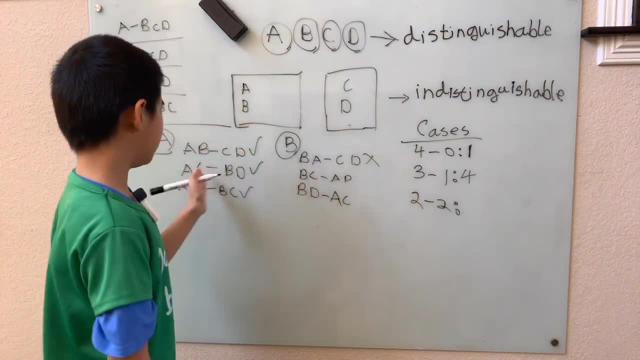 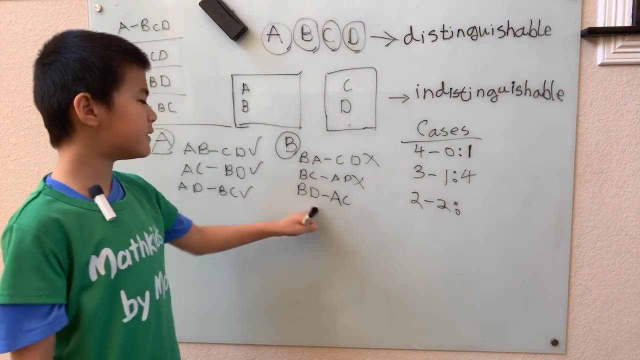 We can't count that possibility. Same with here. we already counted that B C versus A D, we counted that That one's not a possibility. Oh, you're saying with B D A C, B D A C doesn't matter that we swapped the orders. 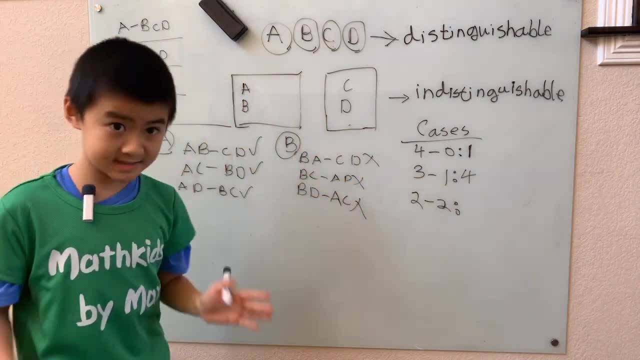 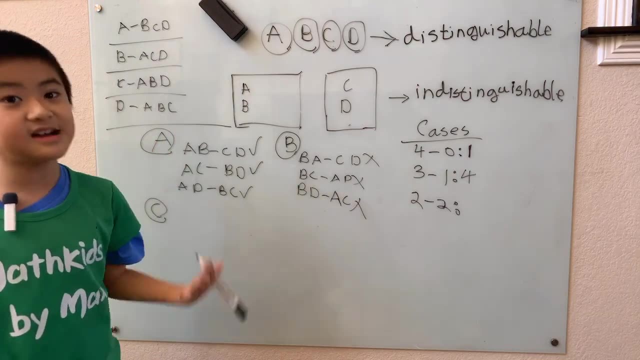 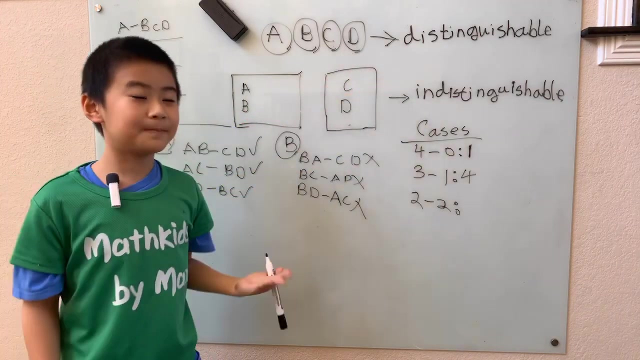 So none of the possibilities when B stays in this box can be counted as another one. So now we want to C. see if we can. C okay, C, C, okay. This is pretty funny, pretty funny. We see if C stays in here and we see if we get any more combinations. 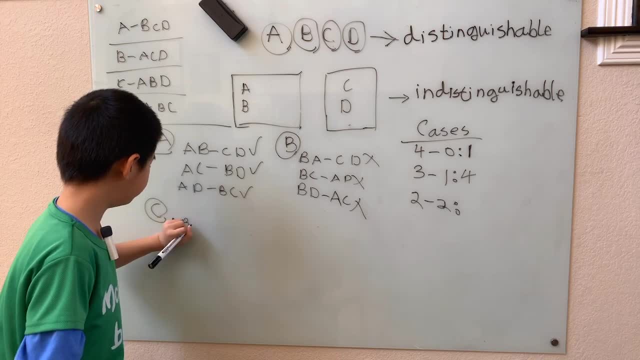 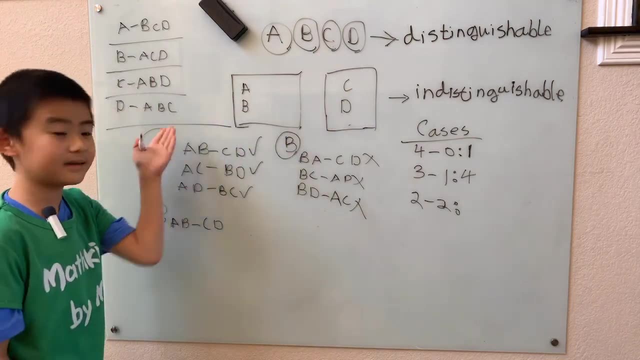 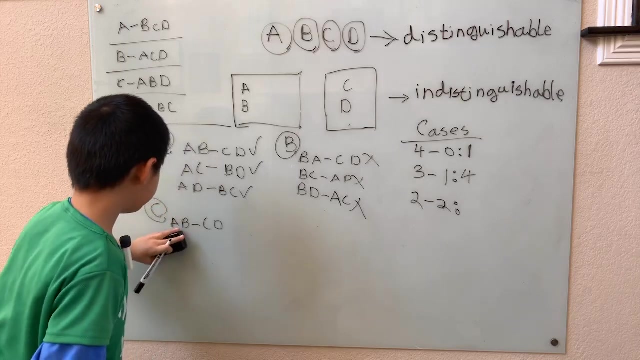 Well, first of all, again we have A, B, C, D, A, B versus C- D. Swap the C and B. I mean the D and A, D and B. I should say D and B to get D, A versus. 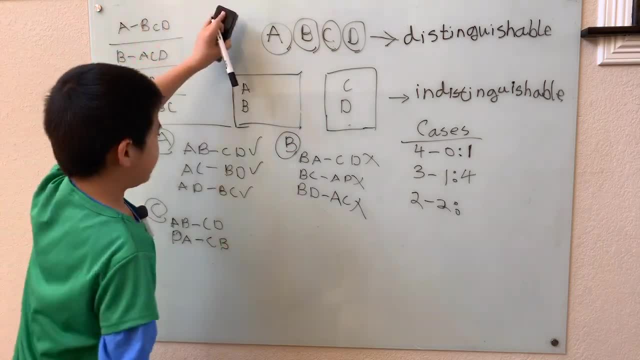 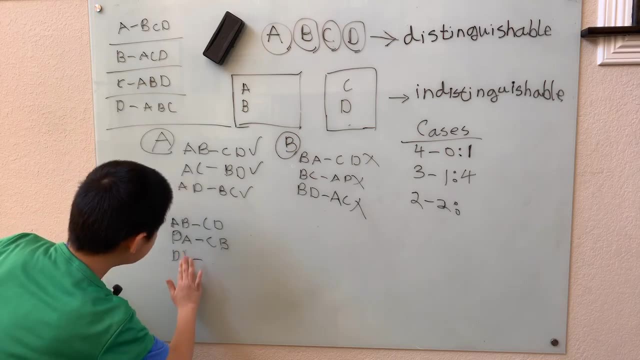 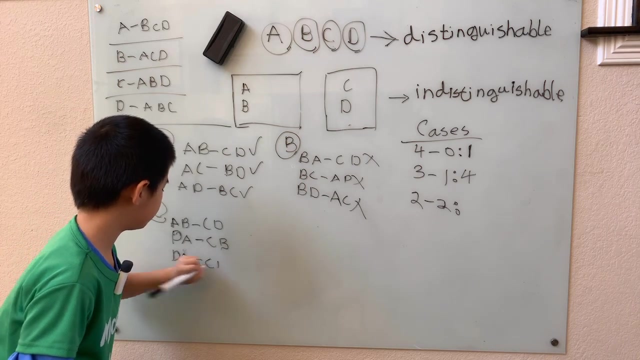 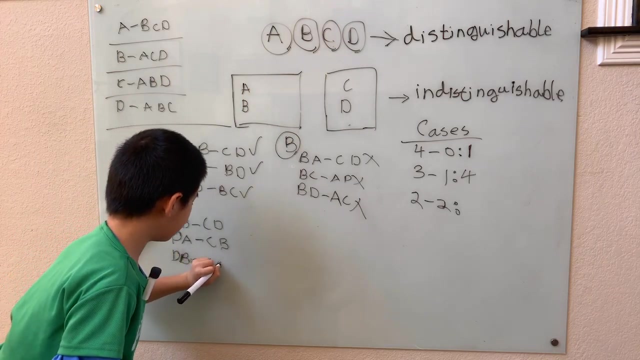 C B and our third and last, combination 2, which will be D A. versus Taking a little time over here, Let me look: D B C A. D B C A. Okay, took a little time there. 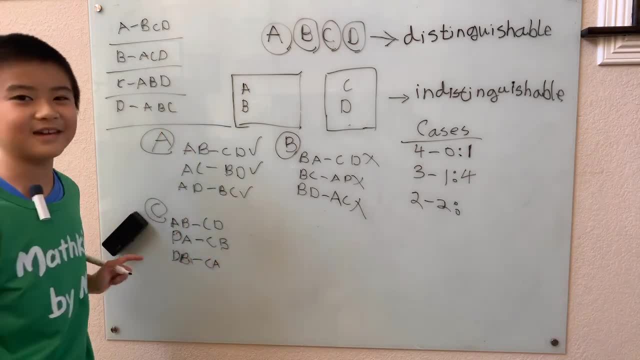 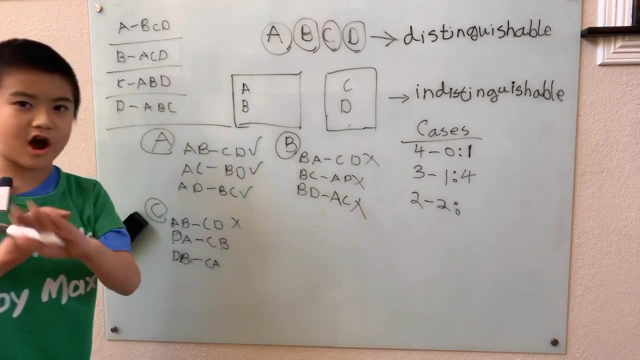 Sorry about the time control, Please don't leave me So again. we see that A, B, C, D. we counted that already. Again, not a combination D A, C, B. Okay, D A stands for Dallas, though. 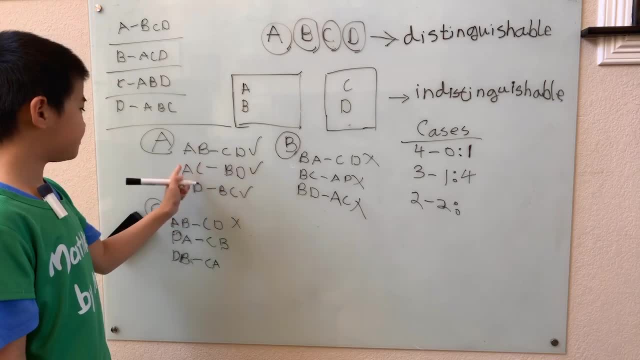 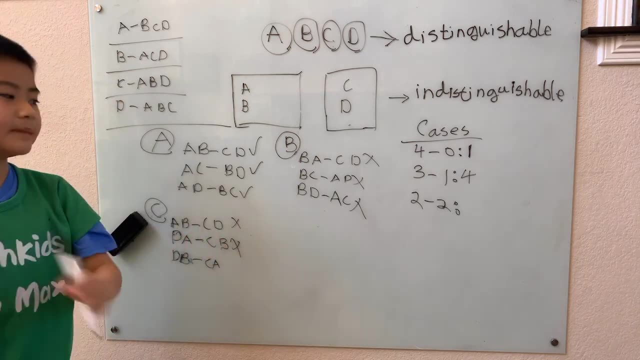 D, A, D, A, D A, C, B, C. B Counted that already. That's a combination. we can't count either, So D. so this doesn't work. Let's start our last one. 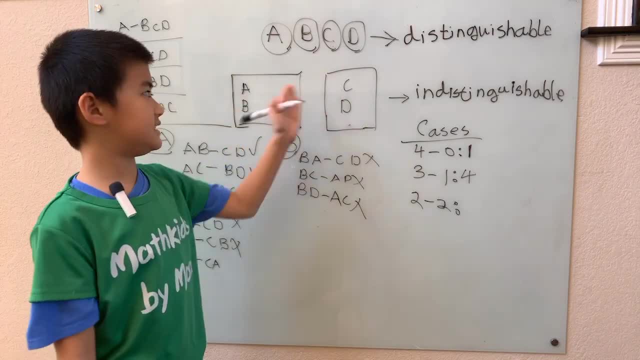 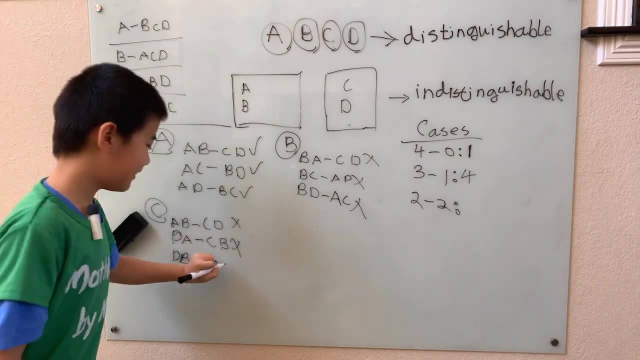 D B and C A, D B C A. I mean, oh sorry, not there. D B C A. counted that already. Now note that we're expecting that our possibilities were D to be correct either. 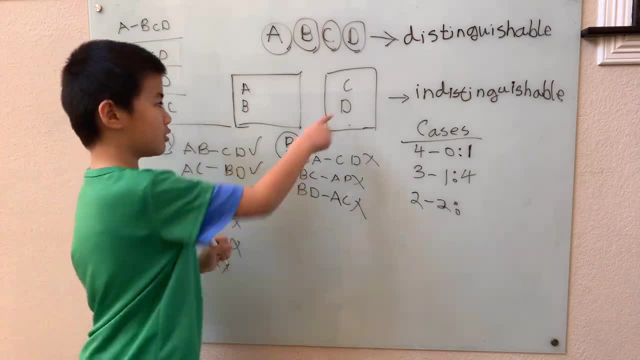 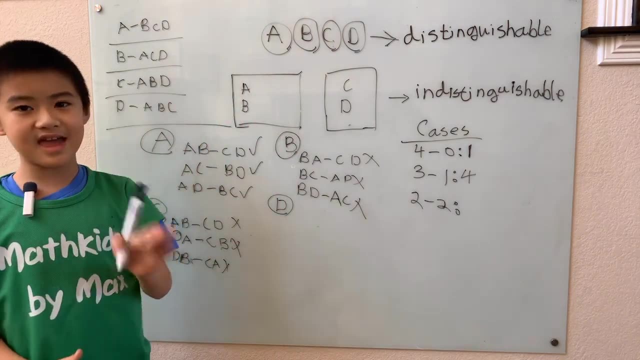 So we're expecting the answer to be three, but just to make sure, we'll check D, See if what happens when D stays. Again see if there is any new possibilities. Okay, and we know: A, B, C, D. 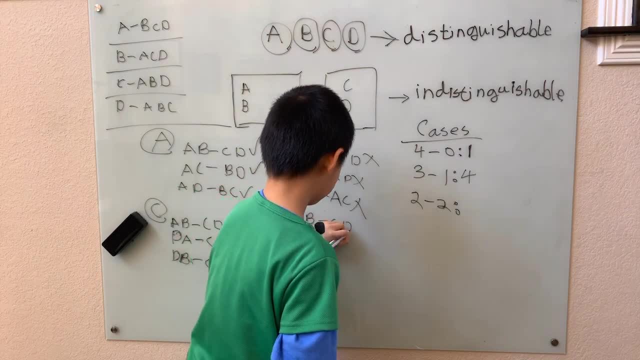 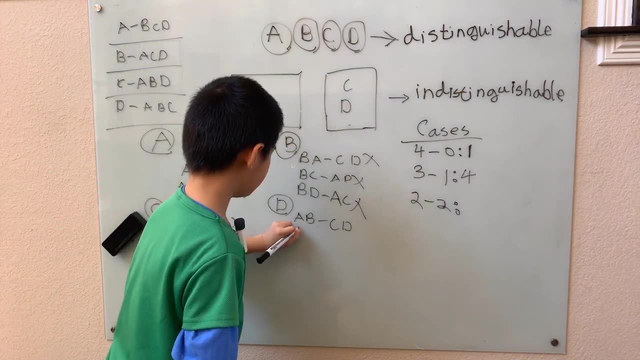 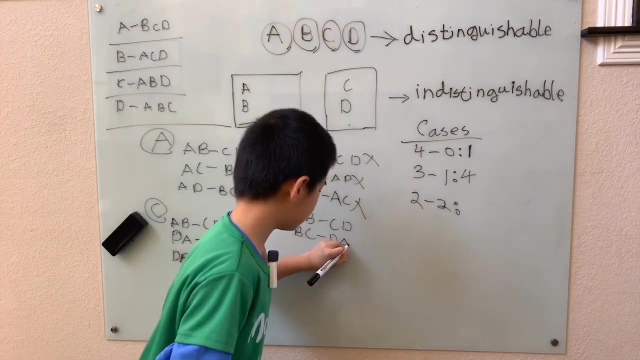 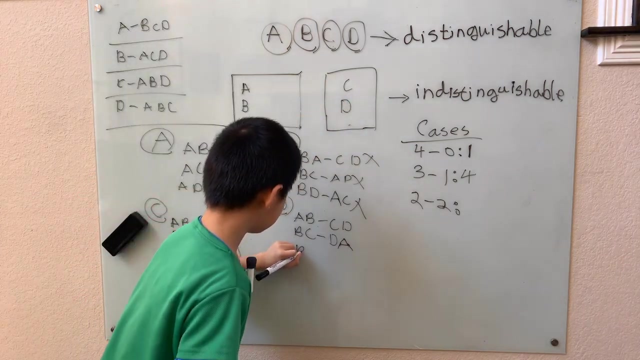 Very old combination. And then we have swapped the C and A to get B? C versus C A. I mean D A, D A, And we got that. We swapped the C with the B to get D B versus C, C A. 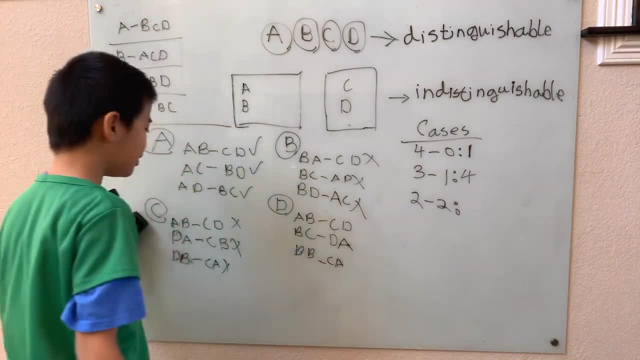 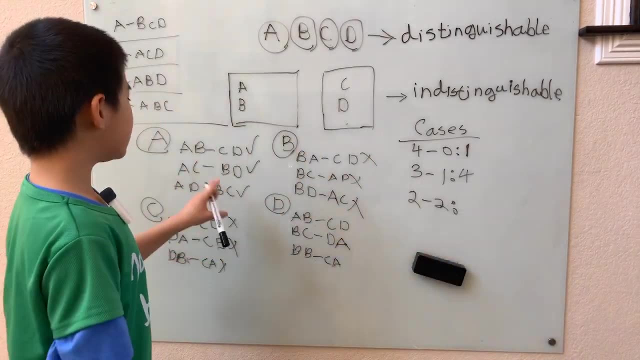 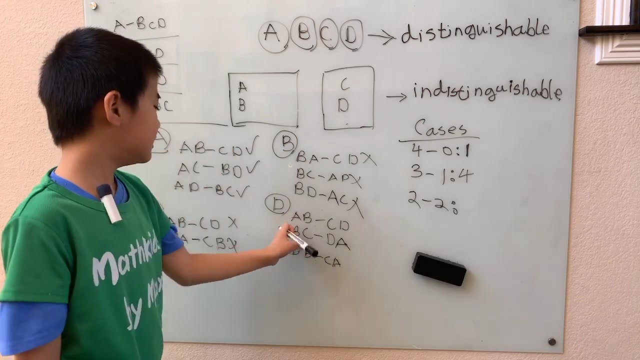 And now we look at if any of these are new combinations. Okay, probably not, but we'll check again. Well, D B looking for D B A. Okay, well, we counted this one already. I I B, C, D, B, C, D A. 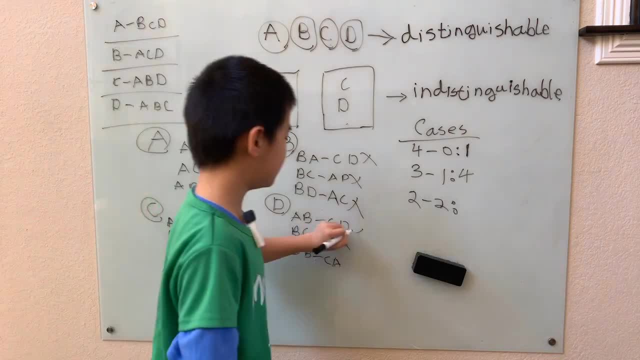 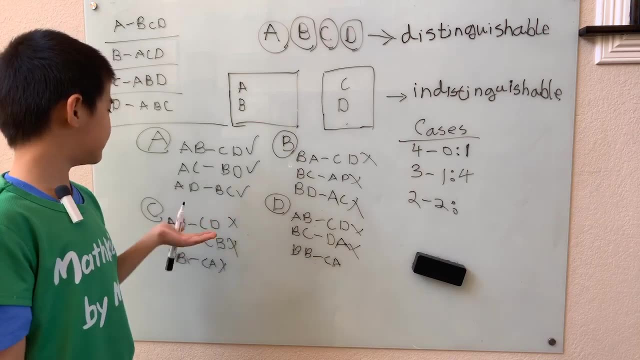 Well, B, C, D A counted out two. So these two got out one final one. See if they'll get us up to four. D, B, I mean B, D same thing. B, D got that. C A counted that already. 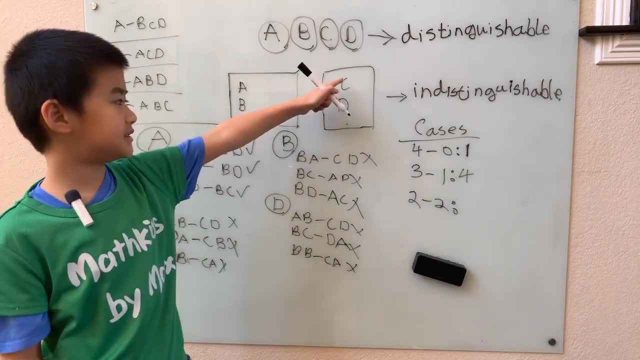 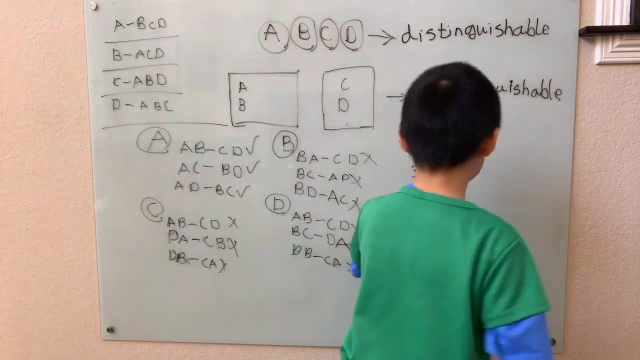 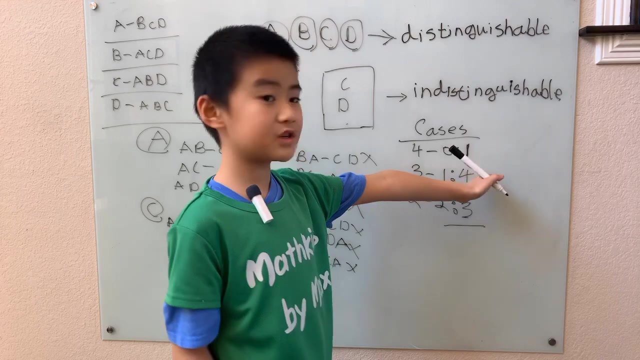 That means none of the B stay, C stay or D stay. none of those will work. So we only have to check A, that's one, two, three possibilities, And just add these up. five plus three, I mean one plus four, is five, five plus three is eight. 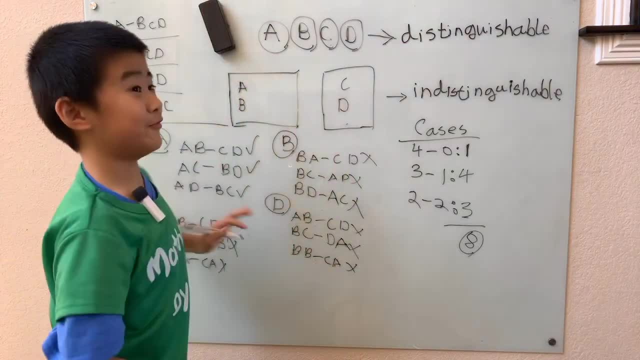 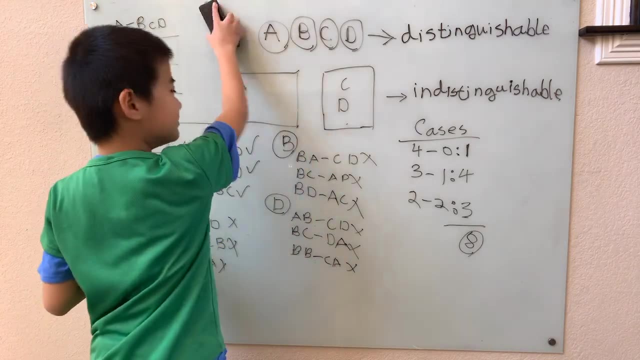 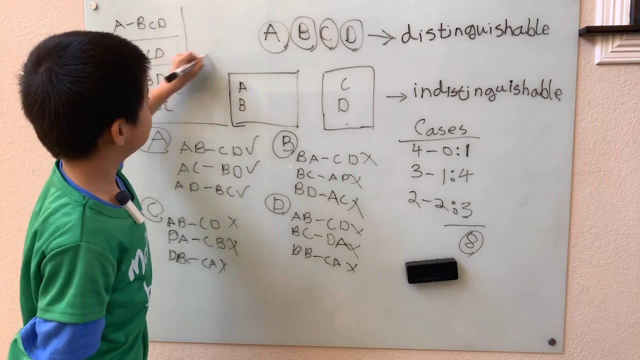 Okay now, after all this computing, we have already forgot that there was an easy way to solve this problem without all this like case work and stuff like that, And of course, we only need this little space to solve this problem seriously. That's how much space we need. 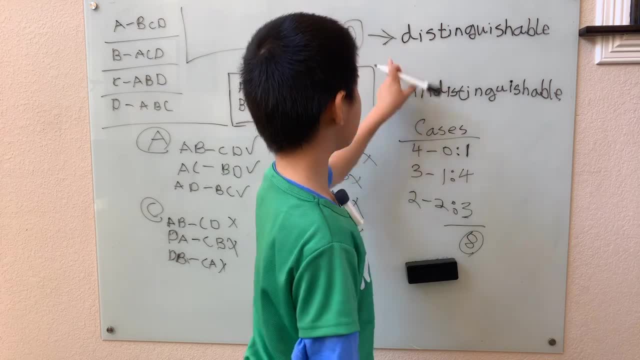 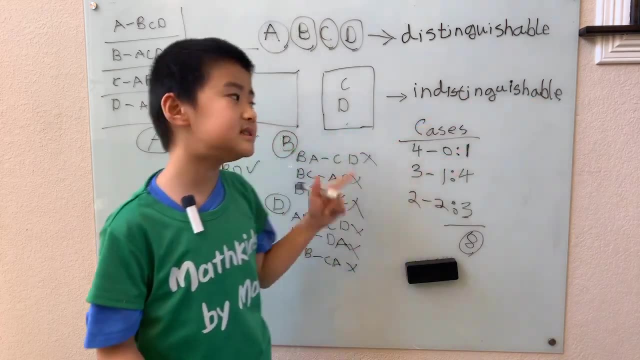 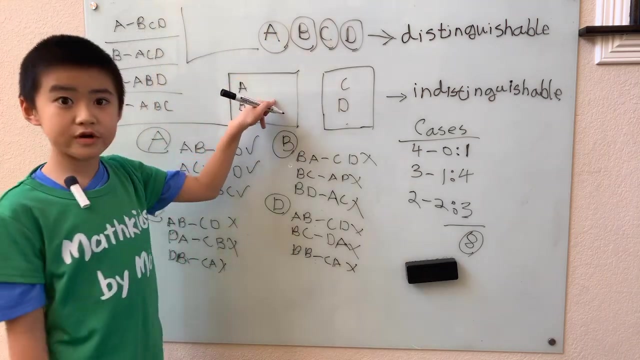 Well, we first look at what happens when all of these are distinguishable, When the four balls are distinguishable, and so are the boxes. The boxes are distinguishable instead of indistinguishable. Well, that would have two balls. I mean two choices for the first one. 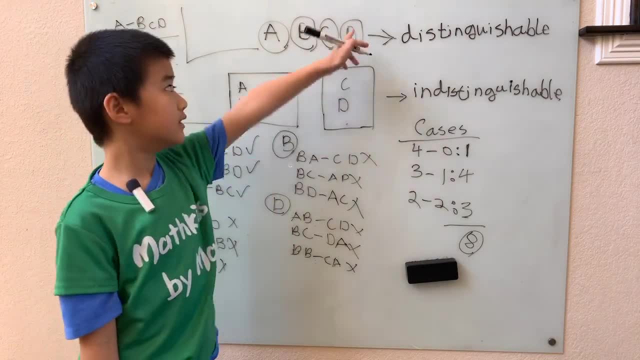 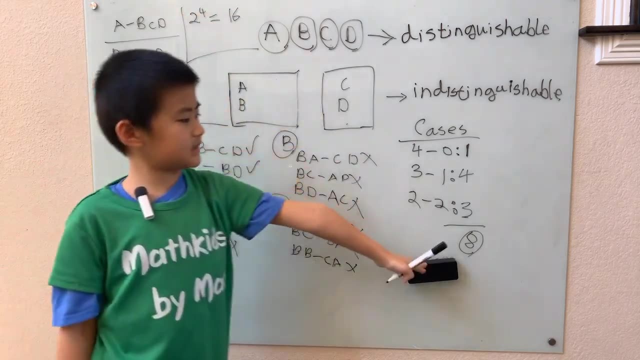 two choices for the second one, two choices for the third one, two choices for the fourth one. Two to the fourth, which equals 16, but 16 is not equal to eight. But why? Because this is when the boxes are distinguishable.